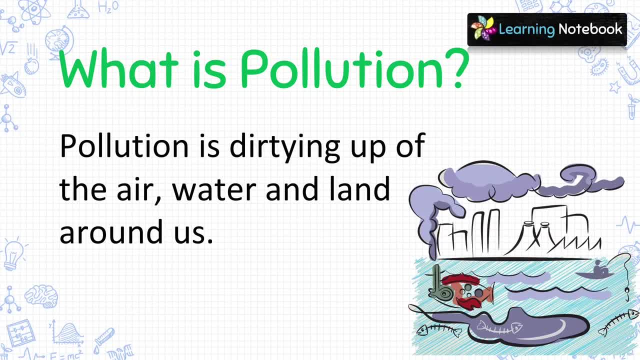 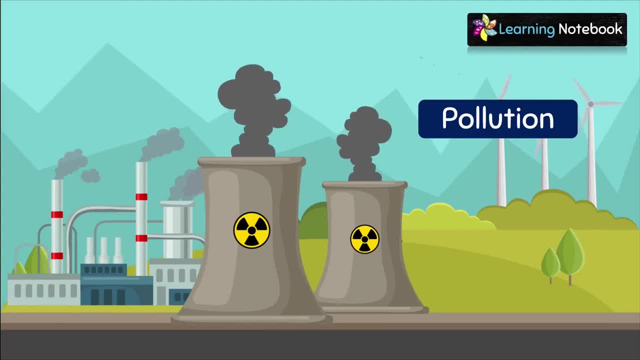 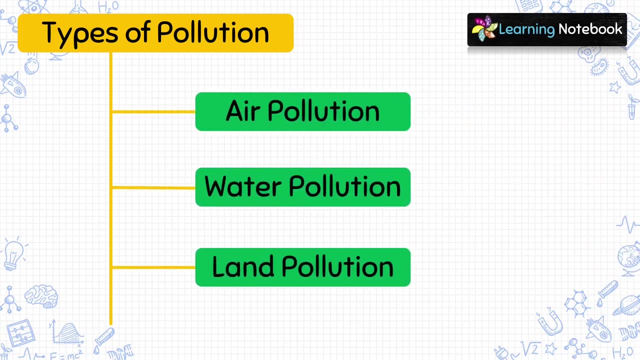 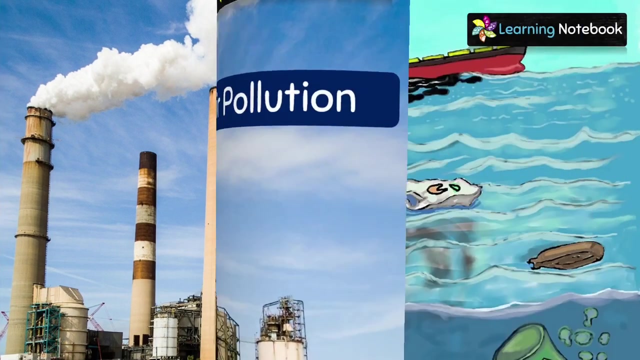 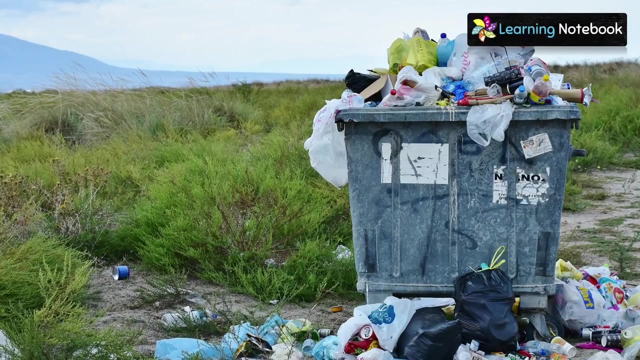 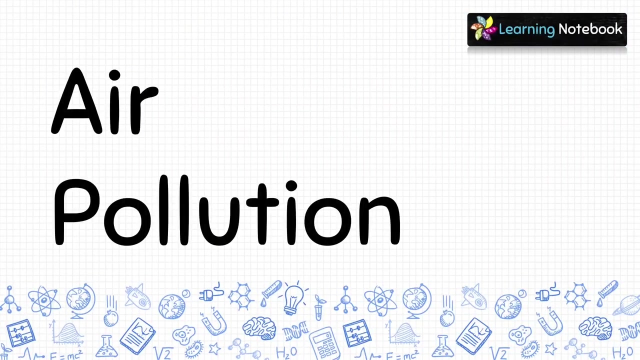 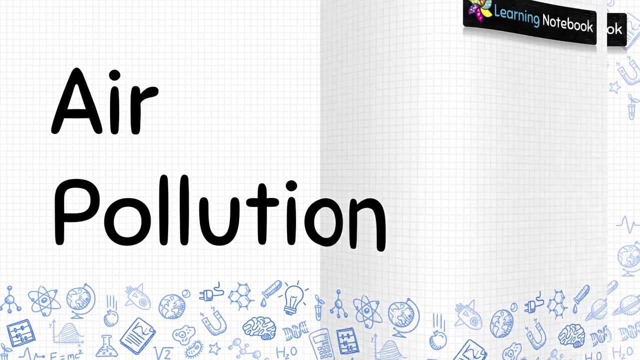 air, water and land around us. And how does this happen? This happens when harmful materials get mixed up with the fresh air, water and land. Three major types of pollution are air pollution, water pollution and land or soil pollution. And first understand what is air pollution: Mixing up of pollutants. What are pollutants? 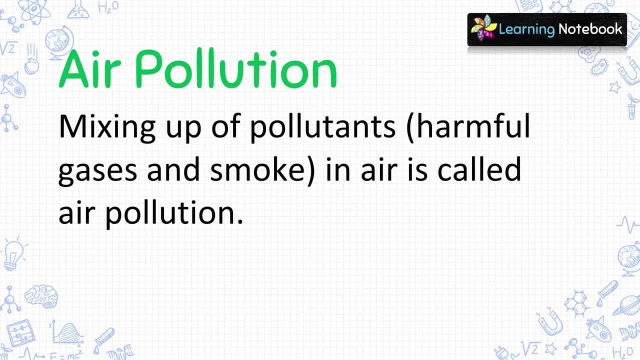 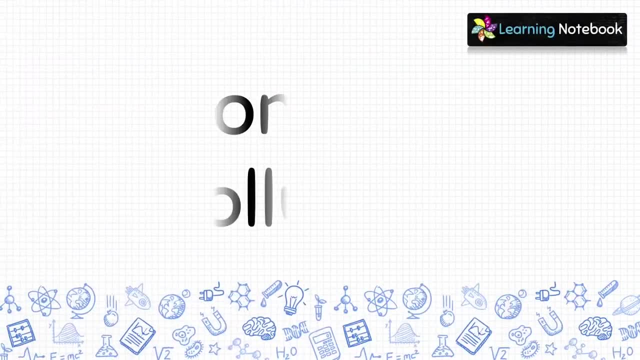 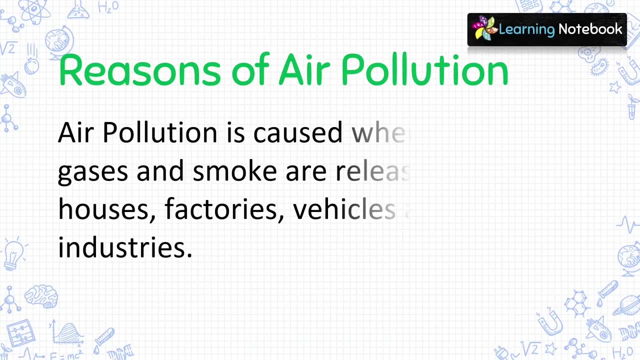 Harmful gases and smoke. So mixing up of pollutants in the air is called air pollution. And what are the reasons of air pollution? Let's see. Air pollution is when harmful gases and smoke are released from houses, factories, vehicles and industries. 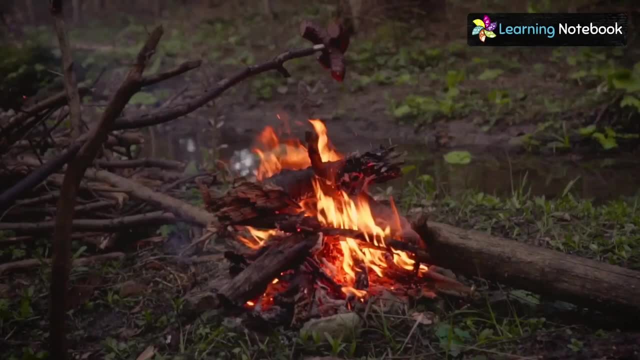 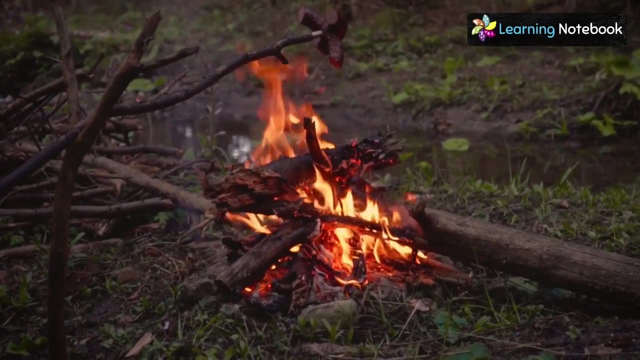 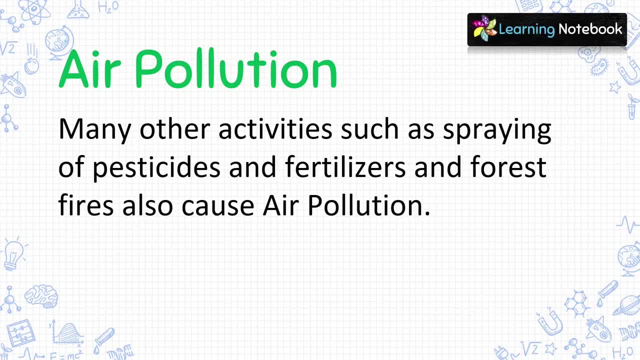 Next reason is burning of wood, solid waste and fossil fuel like coal, oil and natural gas. Next reason is burning of wood, solid waste and fossil fuel like coal, oil and natural gas. Do you know what is forest fire? Let me show you. 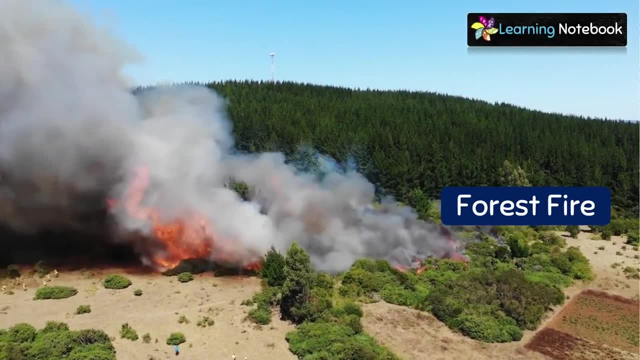 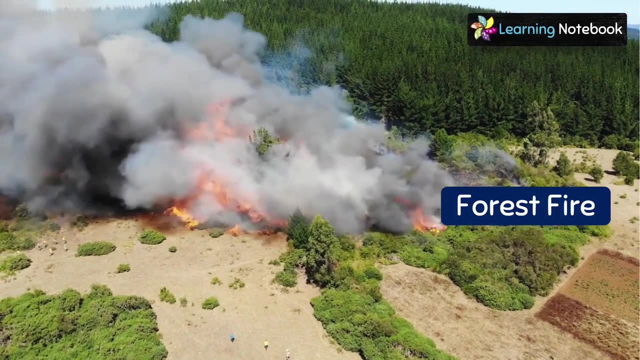 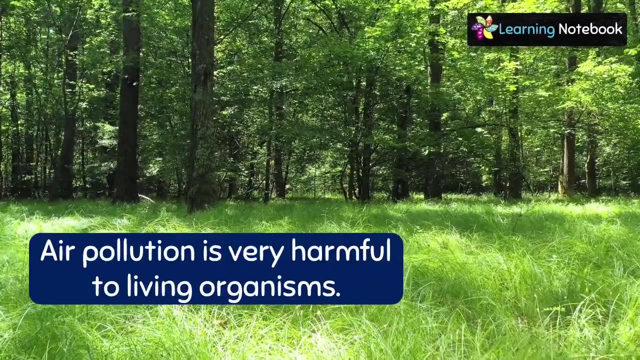 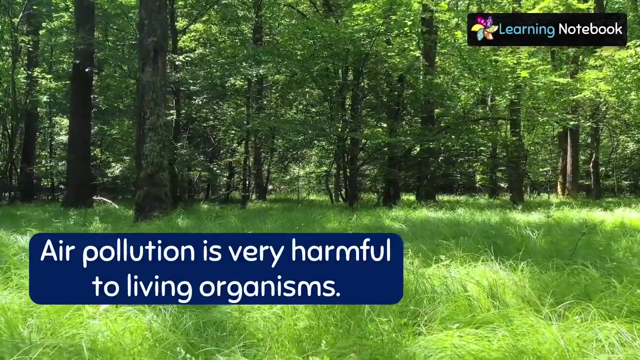 This is forest and feces are getting burned due to fire. See the amount of pollution this forest fire is causing. Air pollution is very harmful and destructive to living organisms. Air pollution is very harmful and destructive to living organisms Because air pollution releases harmful gases. 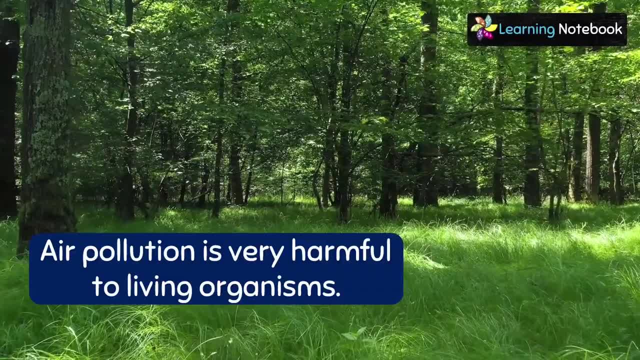 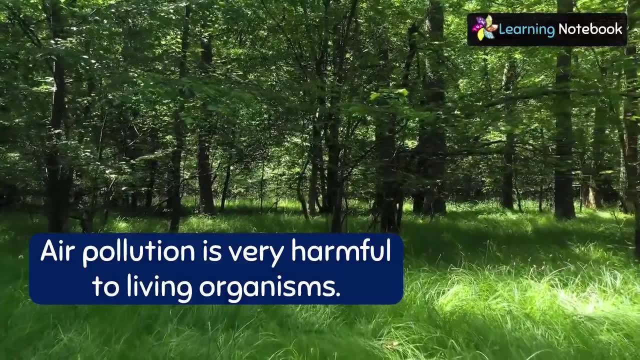 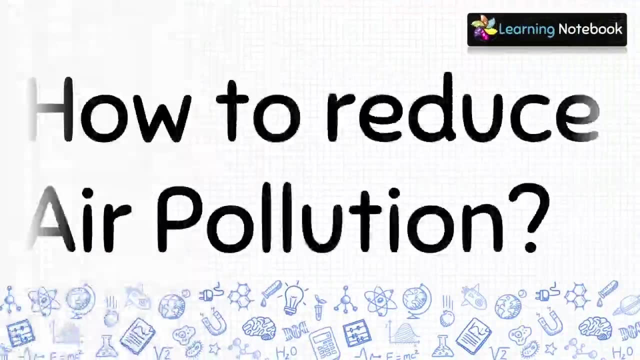 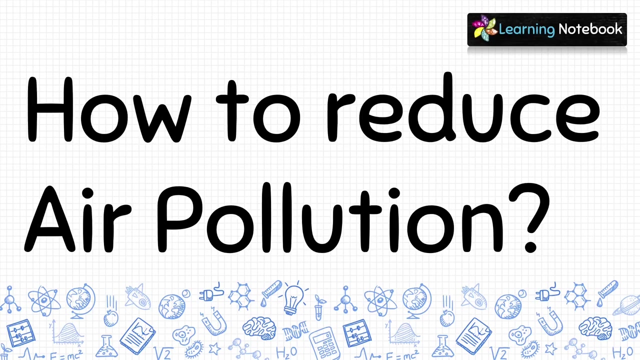 We human beings cause a lot of air pollution. Cutting down of trees increases the pollution level in the air, as trees take in carbon dioxide and release fresh oxygen. So let's understand how to reduce air pollution, Students. air pollution can be reduced if we make a sincere effort to solve this environmental issue. 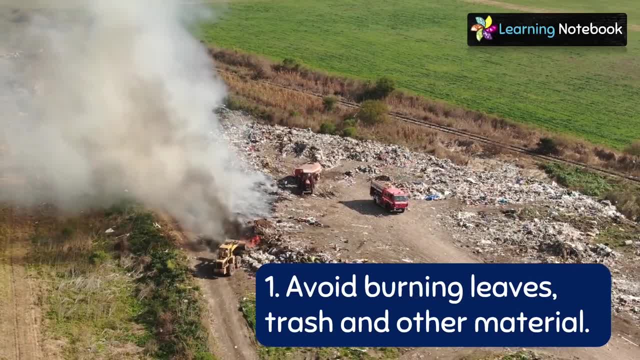 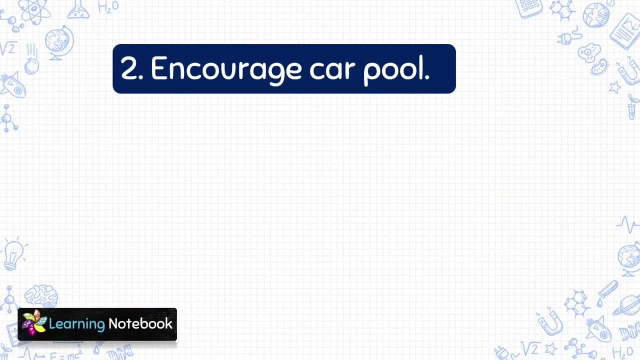 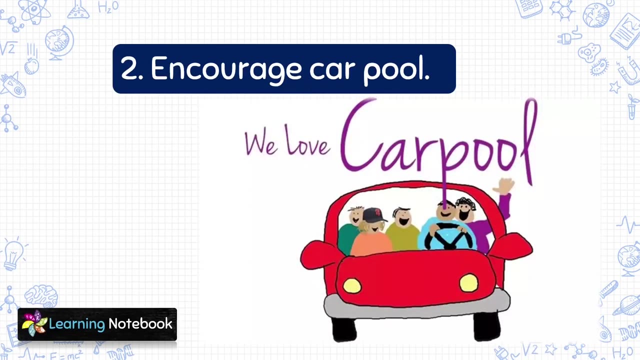 First step is we should avoid burning leaves, trash and other materials. Second, we should encourage carpool so that there is reduction in the number of cars on the road and we can reduce the number of cars on the road And less vehicles lower the level of air pollution. 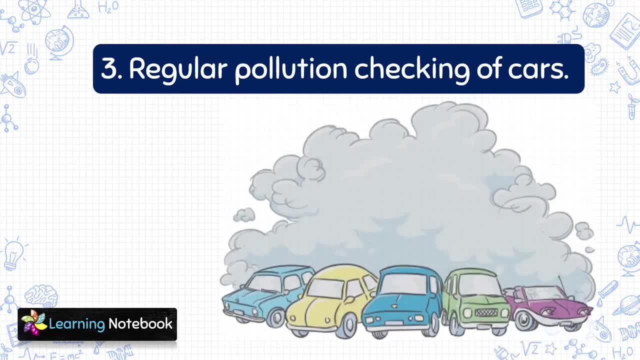 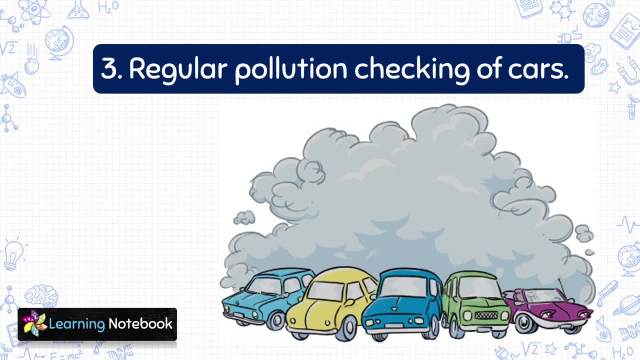 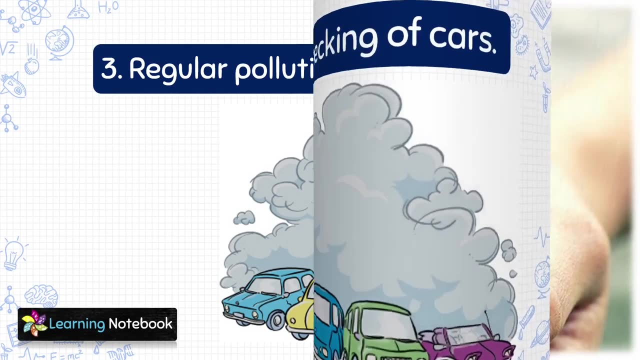 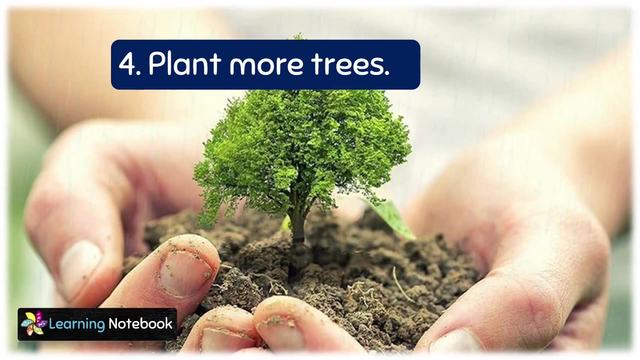 Now third way to reduce air pollution is regular pollution checking of cars. Students cars should be properly maintained and regular pollution checking should be done to avoid air pollution. Now the fourth step to reduce air pollution is plant more trees. We should plant more trees to increase the oxygen level. 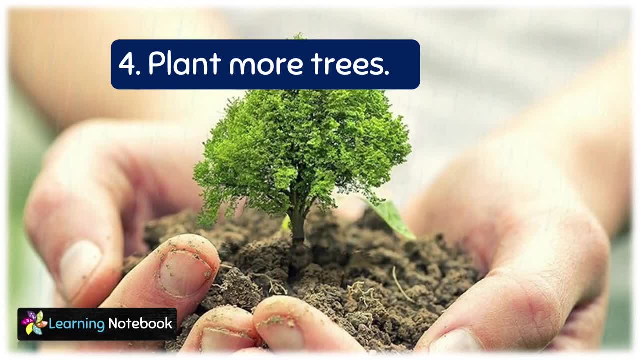 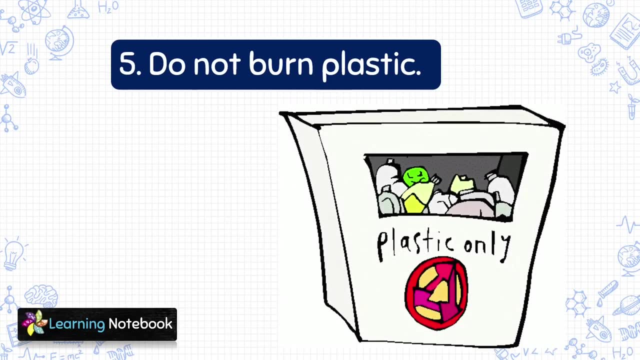 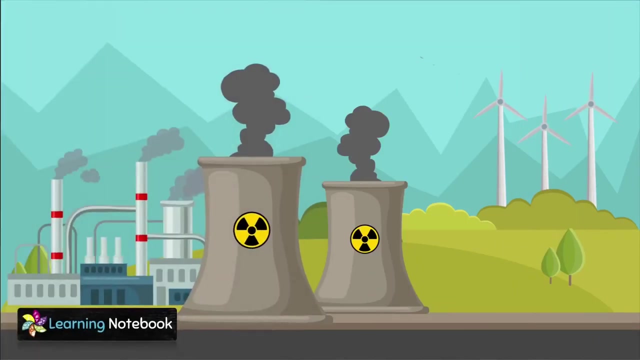 and decrease harmful carbon dioxide in the air. Now next step is: do not burn plastic, Students. we should look to recycle plastic and do not burn it, as its burning causes lot of air pollution. Now sixth step to reduce air pollution is regulate industries. 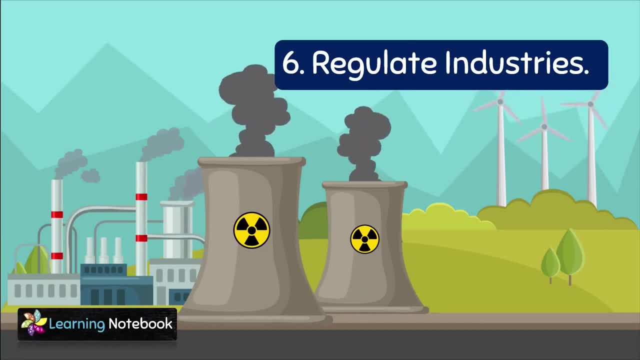 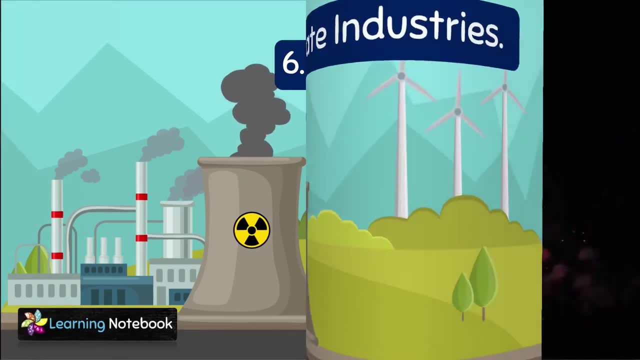 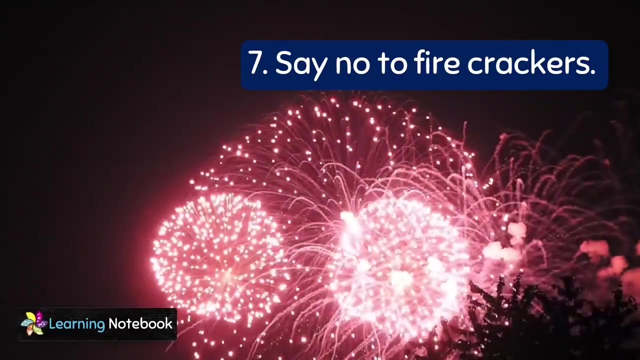 The industries should strictly follow government rules and regulations to control air pollution. And the last step to reduce air pollution is say no to firecrackers. We should not burn crackers as co-reported by the authorities. We should not burn crackers as co-reported by the authorities. 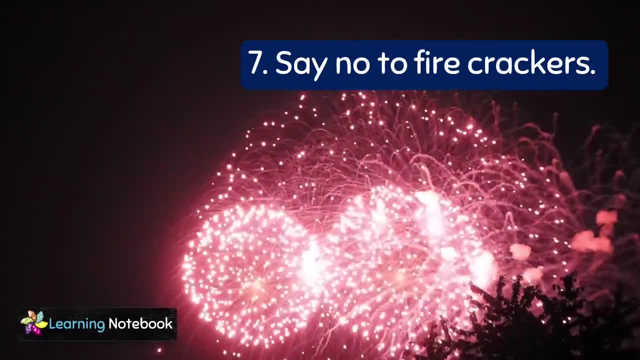 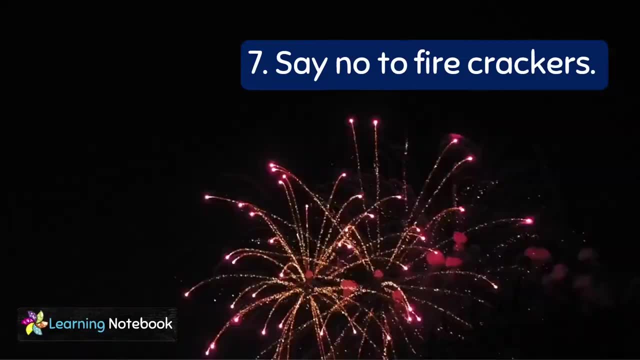 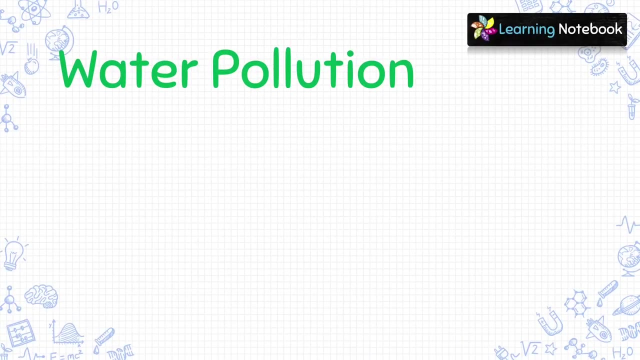 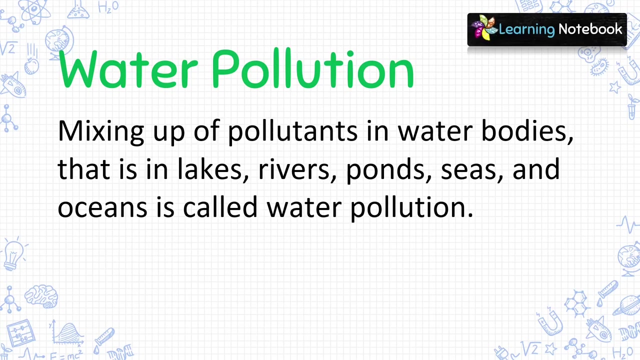 We should not burn crackers. as co-reported by the authorities, it causes a major amount of air pollution. so these were the steps to reduce air pollution. now let's understand water pollution. mixing up of pollutants in water bodies like lakes, rivers, ponds, seas and oceans is called water pollution. 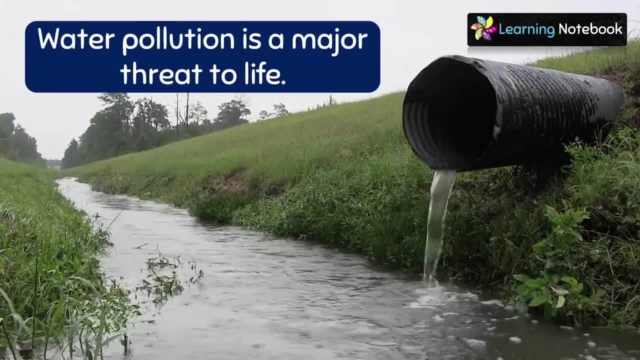 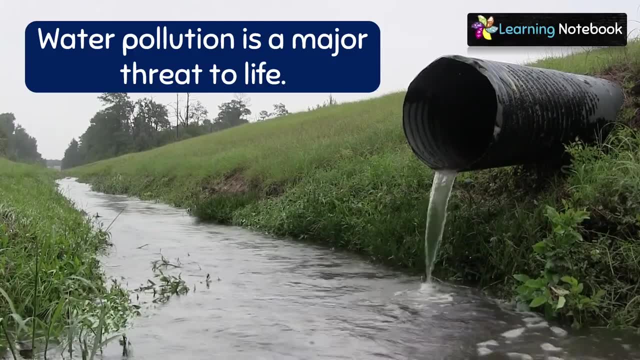 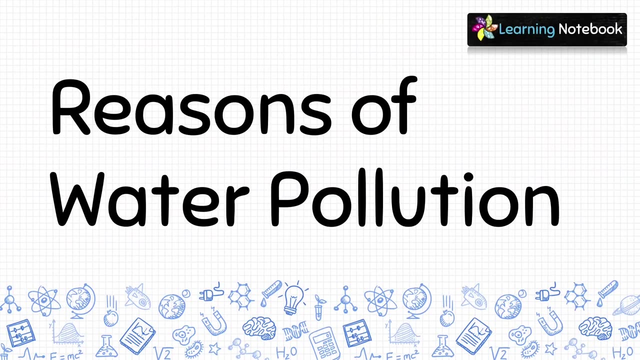 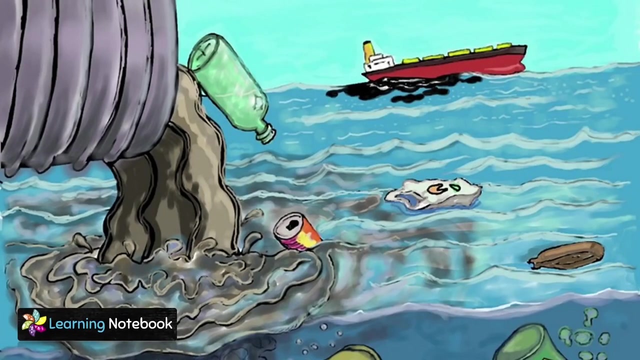 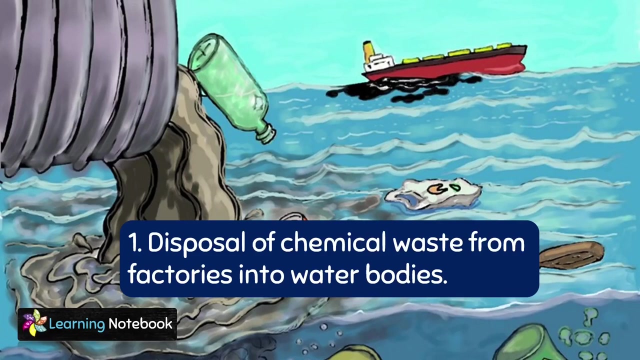 water pollution is a major threat to life. it badly affects the marine life like fishes, crabs, octopus, tortoise, etc. do you know what are the major reasons of water pollution? let's see. first major reason for water pollution is disposal of chemical waste from factories and industries into water bodies. 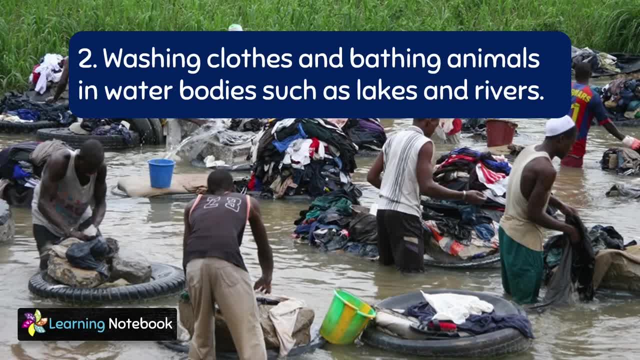 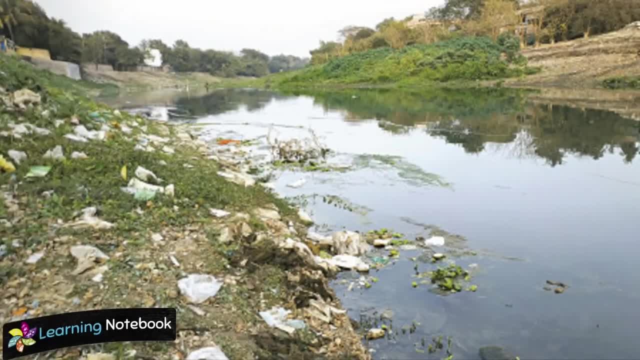 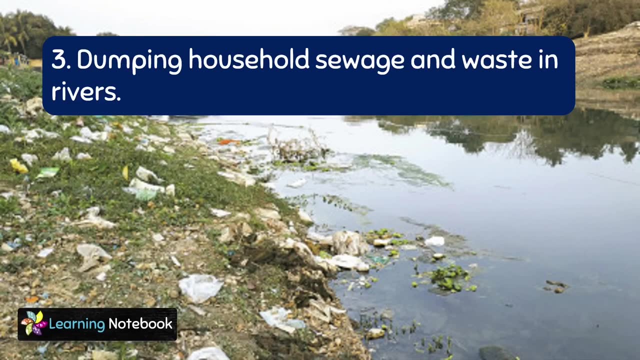 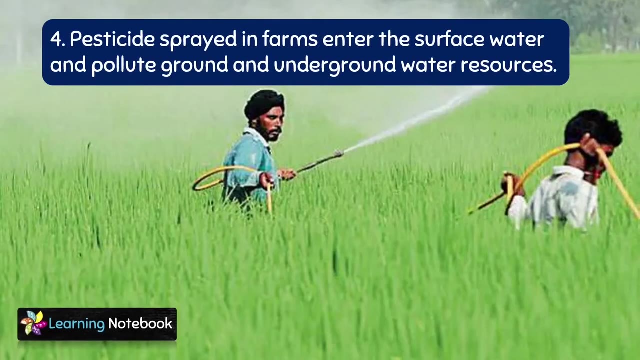 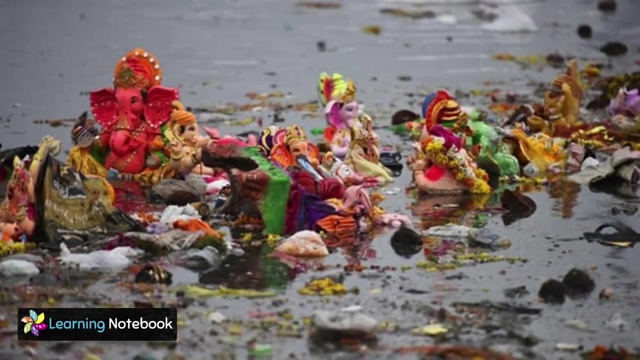 next reason is washing clothes and bathing animals in water bodies such as lakes and rivers. third reason is dumping water running household sewage and waste in rivers. fourth reason is pesticides sprayed in farms. they enter the surface water and pollute ground and underground water resources. and the last major reason for water pollution is idols of god and ashes of the gods. 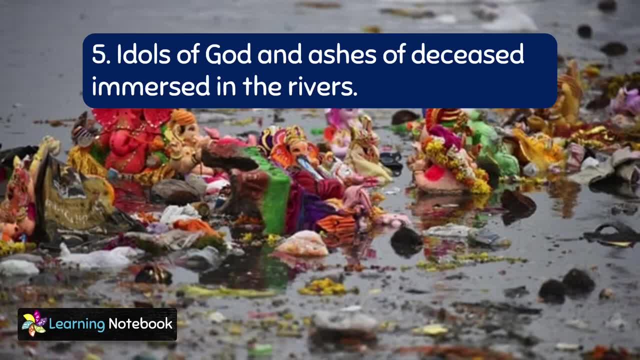 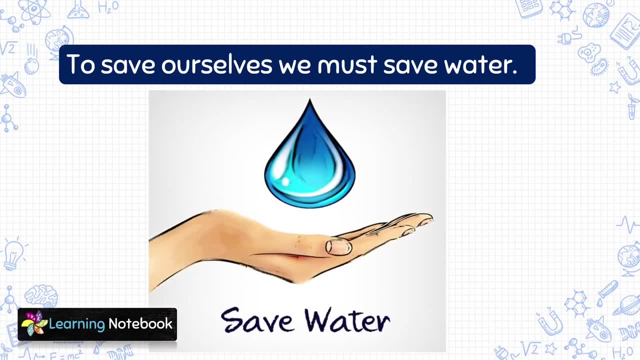 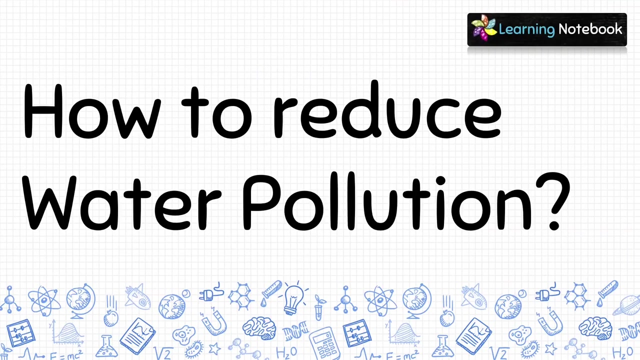 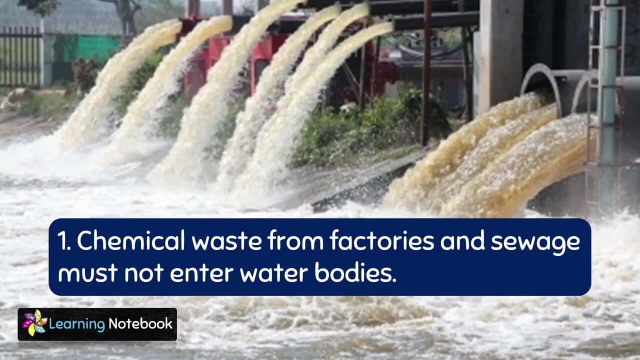 deceased, immersed in the rivers, Students, to save ourselves. we must save water because water is one of the essential resources needed for our survival. Now let's understand how to reduce water pollution. First step to reduce water pollution is that chemical waste from factories and sewage 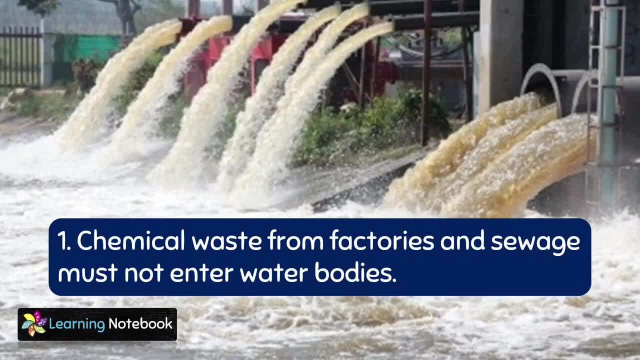 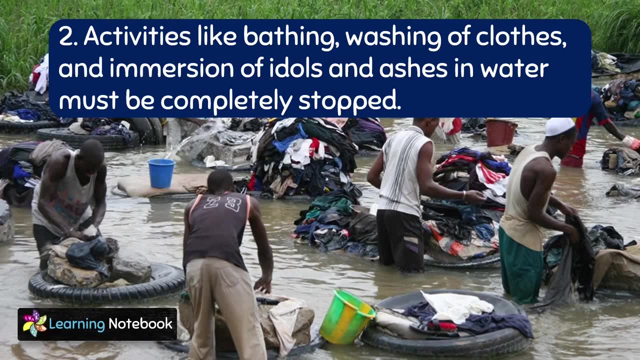 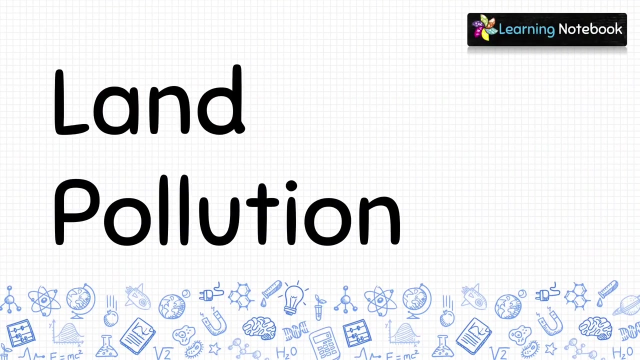 must not enter the water bodies, And then activities like bathing, washing of clothes and immersion of idols and ashes in the water should be completely stopped. So, students, this was all about water pollution. Now let's move and understand land or soil pollution. 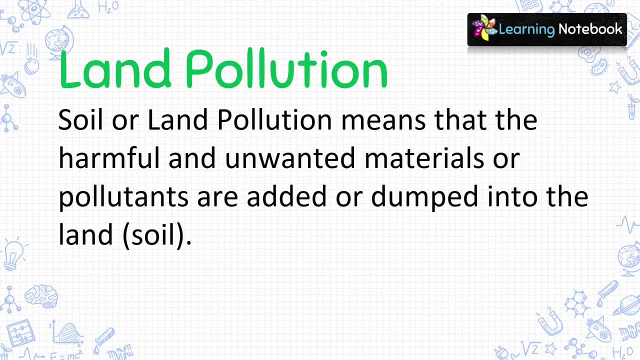 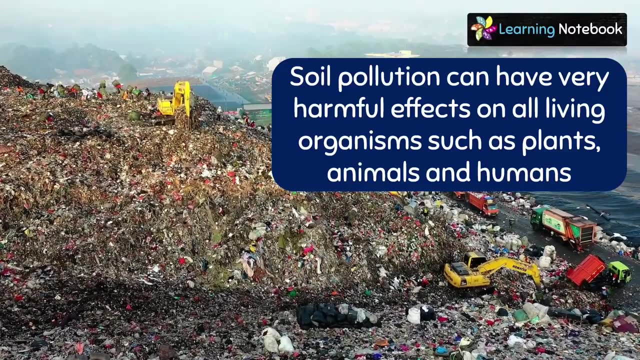 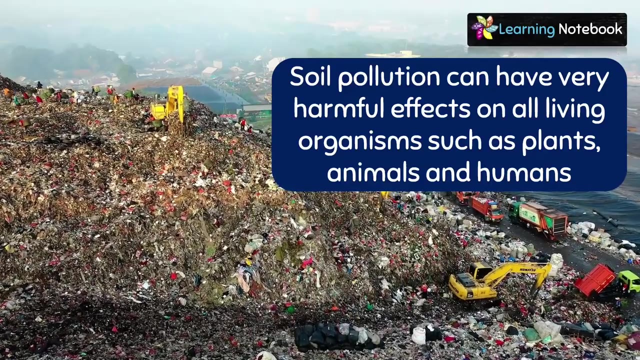 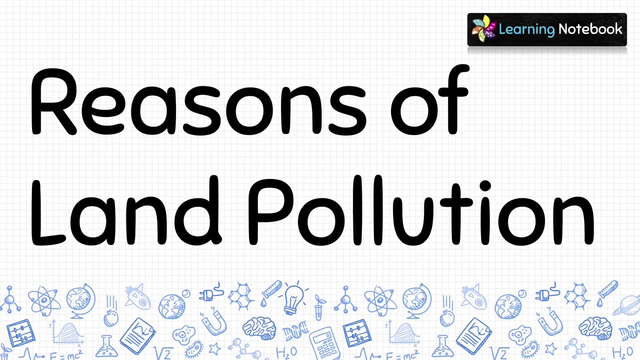 Soil or land pollution means that the harmful and unwanted materials or pollutants are added or dumped into the land. Soil pollution can have very harmful effects on all living organisms, Organisms such as plants, animals and humans. Now let's see what are the reasons of land pollution. 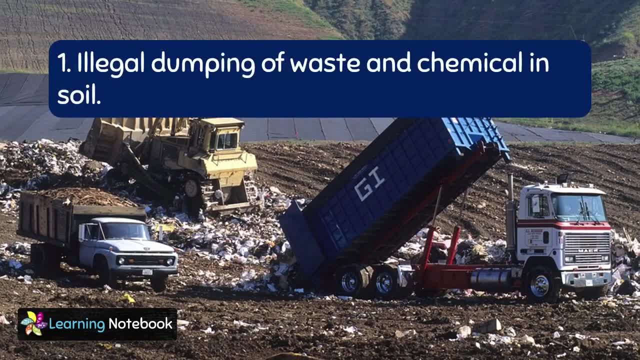 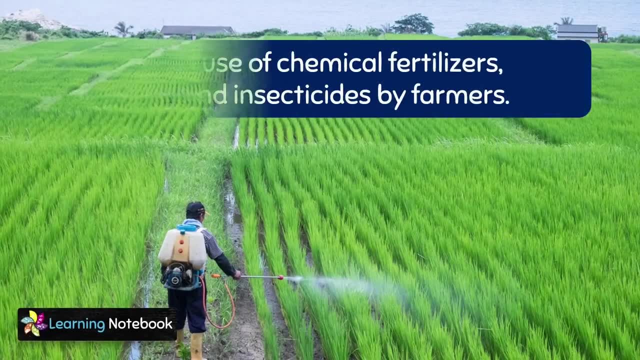 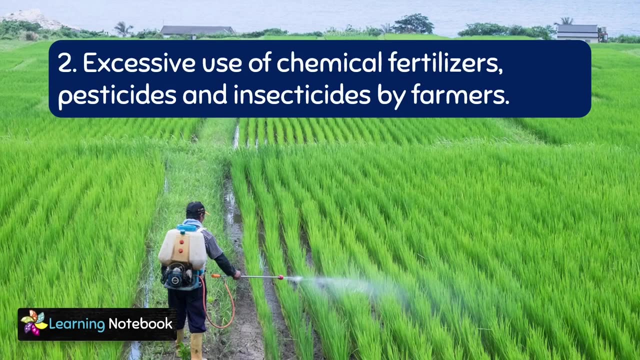 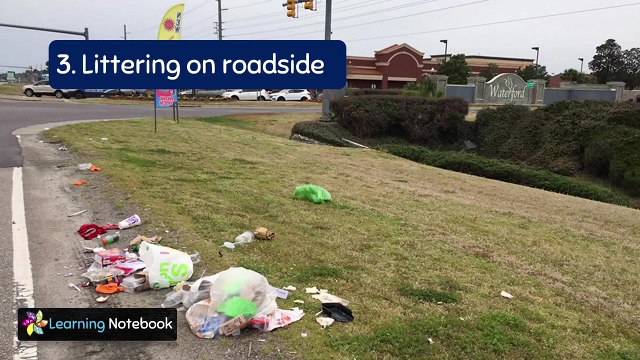 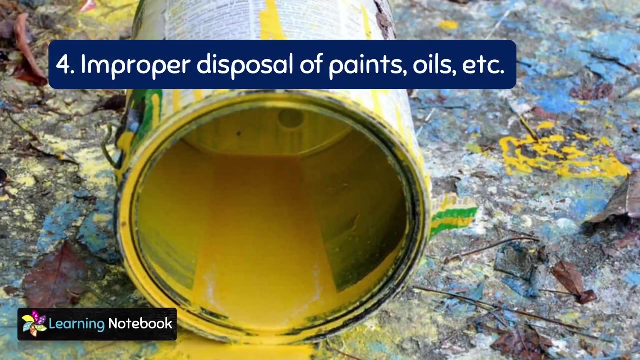 The first major reason for land pollution is illegal dumping of waste and chemical in the soil. Next reason is excessive use of chemicals, Chemical fertilisers, pesticides and insecticides by farmers on their crops. Third reason is littering on roadside. Next major reason for land pollution is: